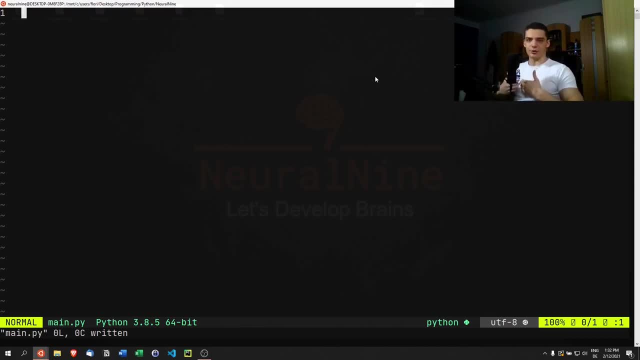 or it uses an additional layer of abstraction, or you could also say protection, when it comes to creating instances of classes, And let's look at an example here. Let's again start by importing from ABC. So from abstract class, we're going to import ABC meta. 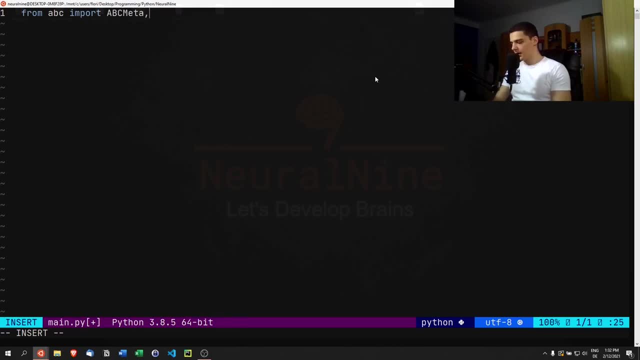 and abstract static method, And then we're going to again create an IPerson interface- IPerson- and we're going to pass, going to pass meta class, ABC, meta, And in here we're just going to have a basic abstract static method And this is just going to again be person method. 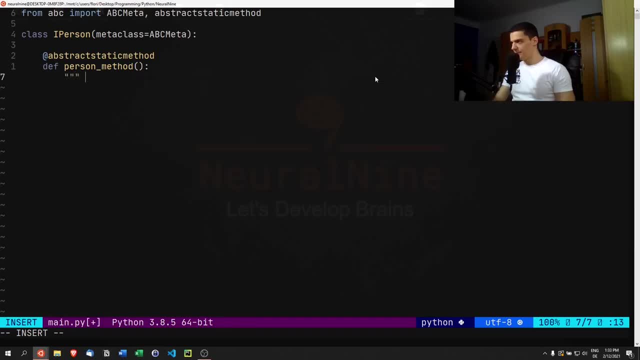 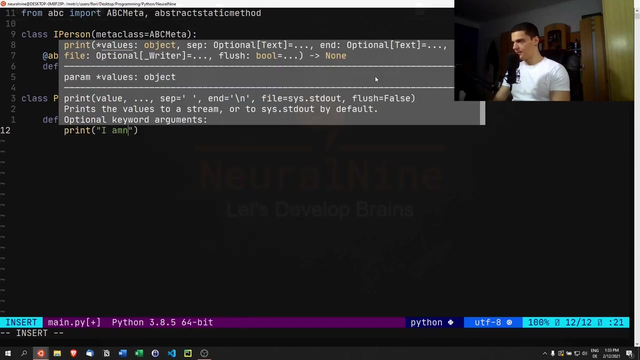 And this person method is just going to be implemented later on, Because this is an interface method. And now we're going to also create a person class which implements the IPerson interface. And here we're going to say: def: person method print. I am a person, So just a basic functionality here And now what we want to do is: we don't want 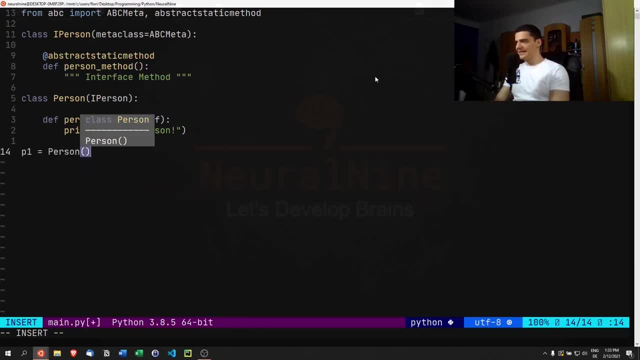 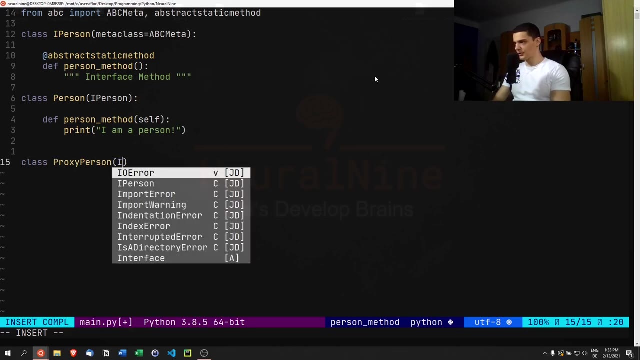 to go ahead and say P1 equals person, because that's too direct of an instantiation. We're going to use a proxy, So a middleman, you could say, to create and handle the person object. So we're going to say class proxy person, which is also going to implement IPerson. 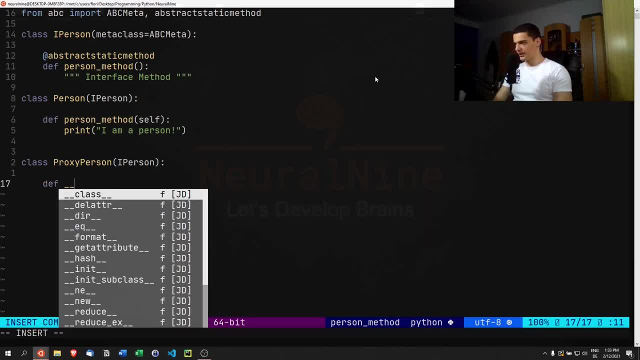 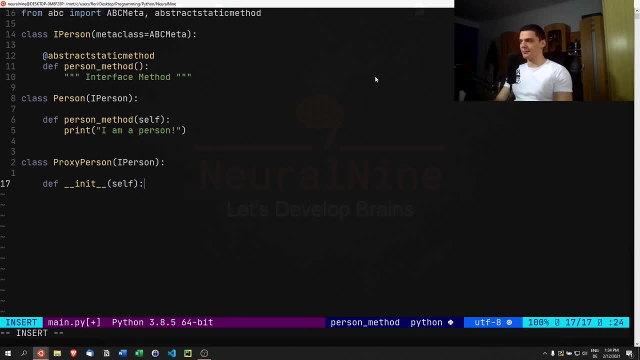 And this class is going to have a constructor. So we're going to say init self: And here we're going to basically create a person instance that we're going to have as the instance that we're going to manage here. So we're going to, whenever we create a 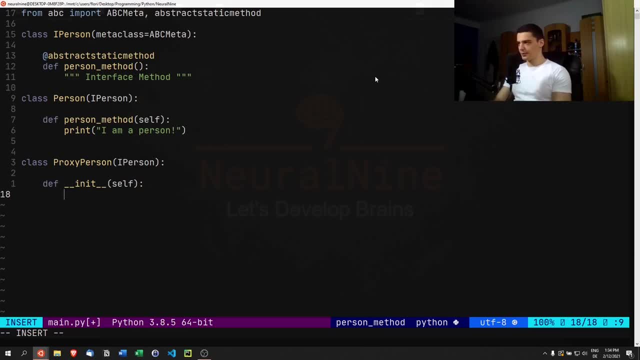 proxy person, we're actually creating an actual person object. So we say selfperson equals person, like that, And this is now the person object that we're going to manage. But whatever, whenever we do something, we're going to also wrap the proxy functionality around it, So we can also have the 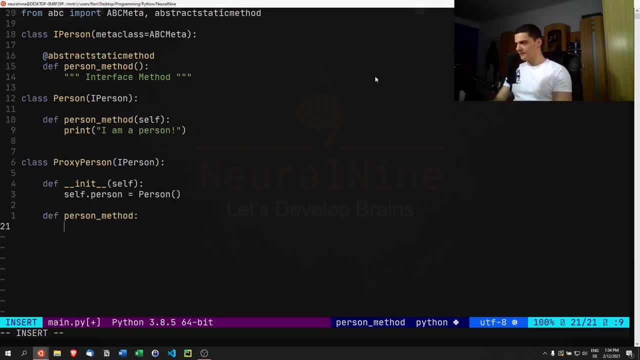 person method here, since we're implementing the IPerson interface And here we're just going to go ahead and say: print, I am the proxy functionality, And here you can actually do whatever you want functionality. And then you can go ahead and say: 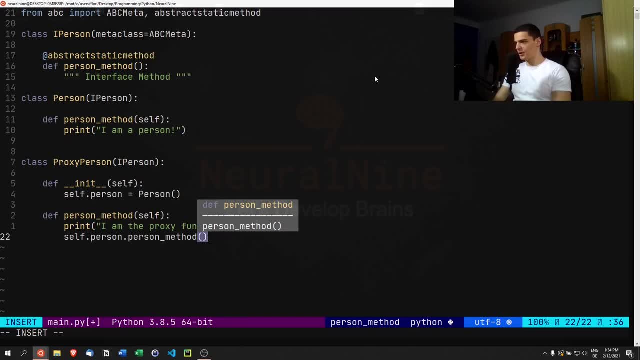 selfpersonperson methods. So here we're calling the actual person method, from the actual person class, from the actual person object, but around it, So before it, after it, we can do whatever we want. you can have logging, you can have timing, you can have whatever you want. This is the, this is where the protection comes in. you control. 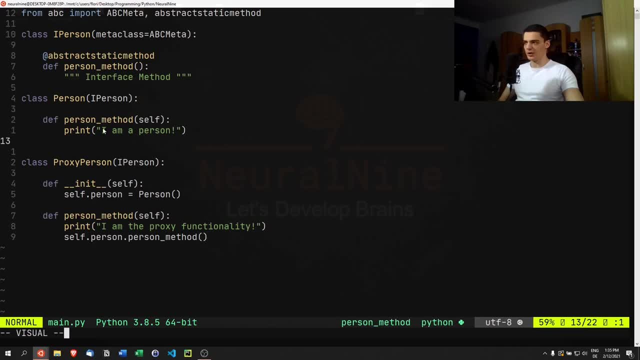 what happens when you call certain methods. So you're not just creating a proxy, A person object, and creating it directly and managing it and and calling the functions directly. you have this proxy middleman class that adds its own functionality. When you call a method, when you create it, you can also add some. 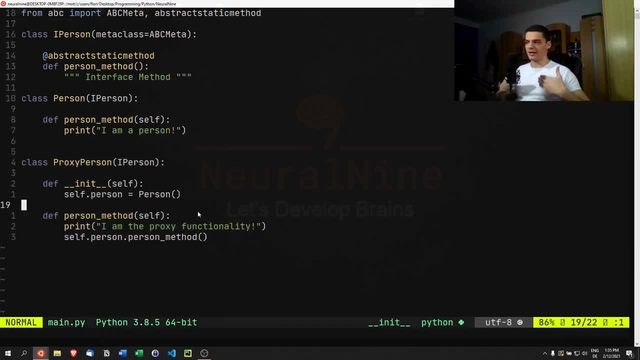 functionality here in the constructor so that you have this layer of abstraction and protection And it just gives you more control and more encapsulation when creating person objects. So you can see, actually when I go ahead and say p one equals person, not permission error person, And then p one person methods, we get one functionality. And if I go ahead and say p two, 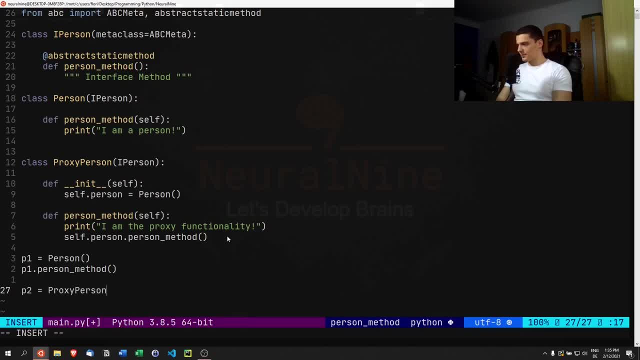 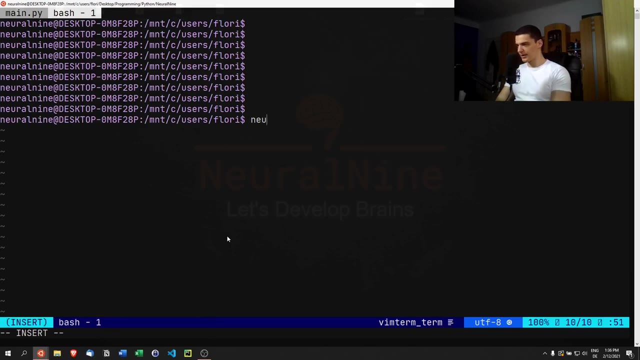 equals proxy person. proxy person, p. two person method. we're going to get different outputs. So let me just open up the terminal terminal tab, bash, let me just go down a bit so that I'm not blocking again with my camera, and then Python. 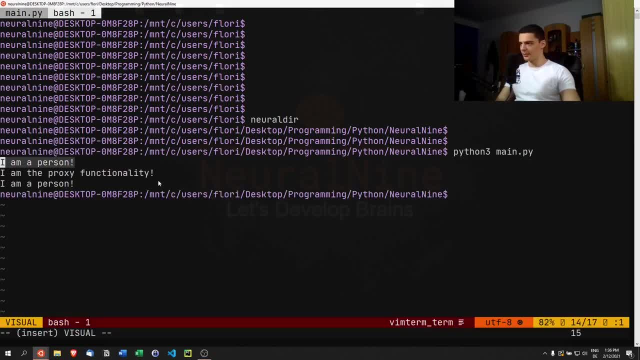 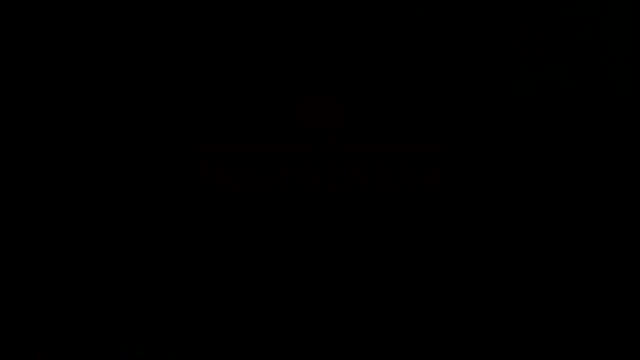 three main py and you're going to see I'm the person or I'm a person, And then we get the same thing with the proxy functionality And that's the basic idea of the proxy design pattern. So that's it for this video. Hope you enjoyed it. 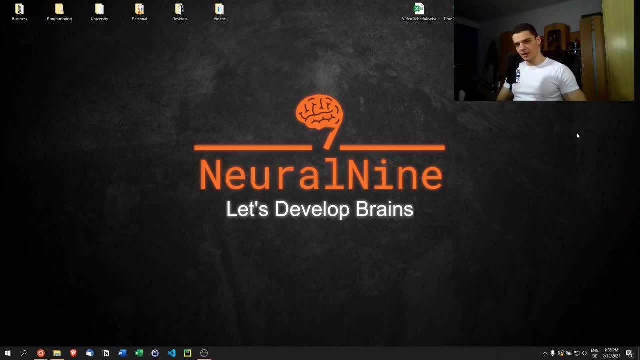 I hope you learned something. If so, let me know by hitting the like button, leaving a comment in the comment section down below. And, of course, don't forget to subscribe to this channel and hit the notification bell to not miss a single future. 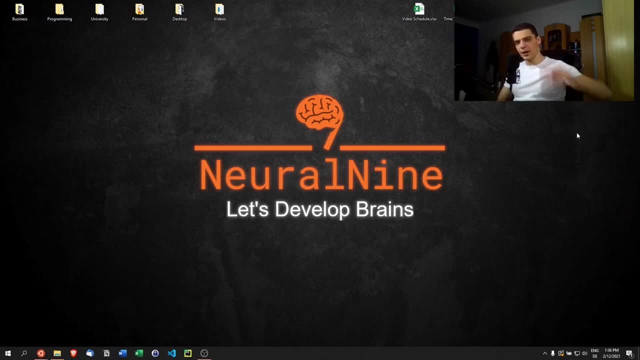 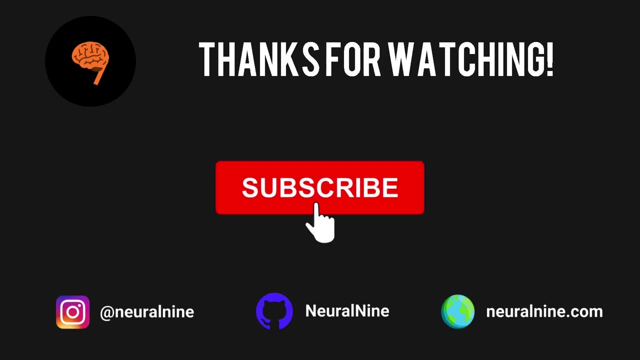 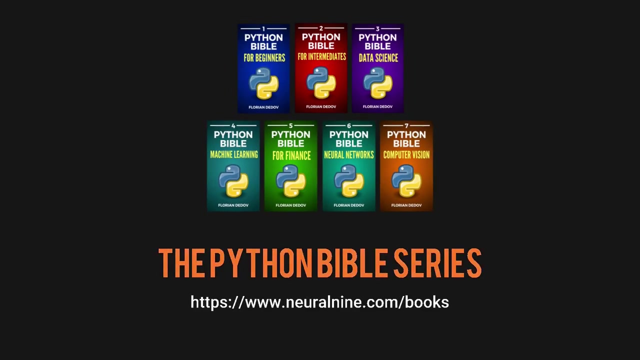 video for free. Other than that, thank you very much for watching. See you in the next video and bye, bye.